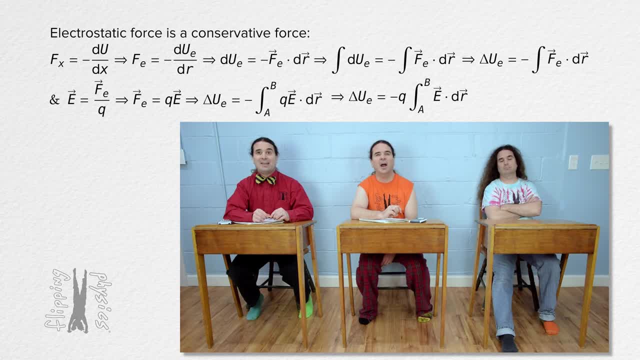 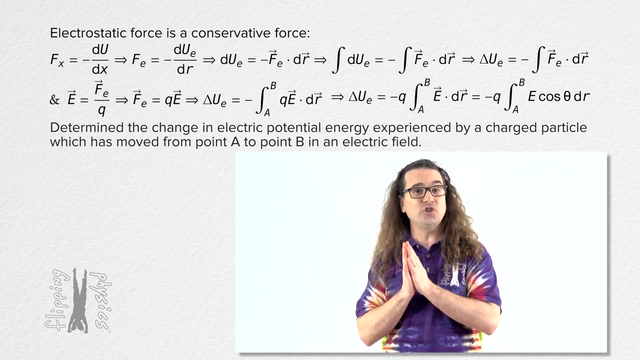 charge out from under the integral And we can have either the dot product version of the equation or the one without vectors and the cosine of the angle between the direction of the electric field and displacement dr instead of vectors. Well done, Billy. We have now determined the change in electric potential energy experienced by a. 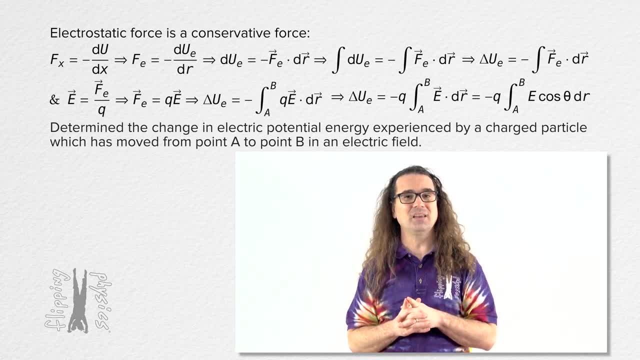 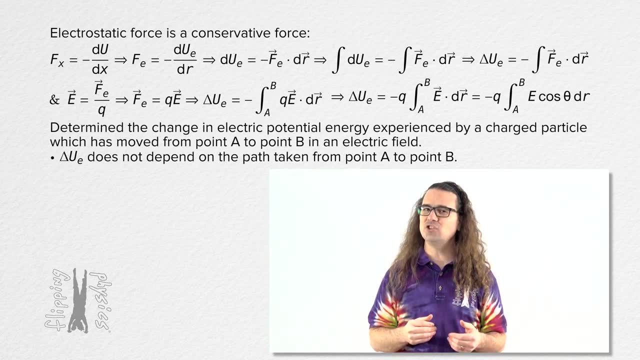 charged particle which has moved from point A to point B in an electric field. Notice, because the electrostatic force is a conservative force, this change in electric potential energy does not depend on the power of the electric field on the path taken from point A to point B. 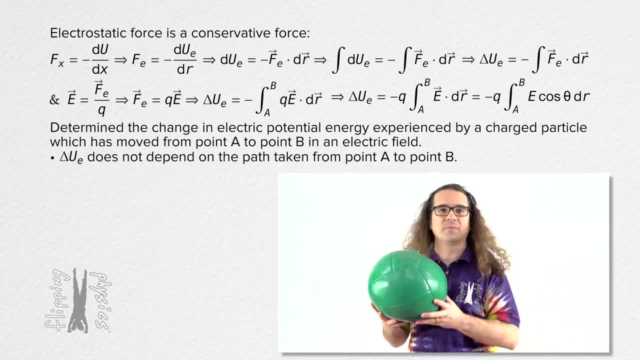 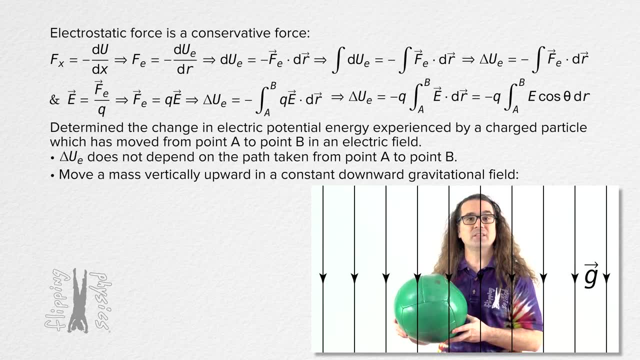 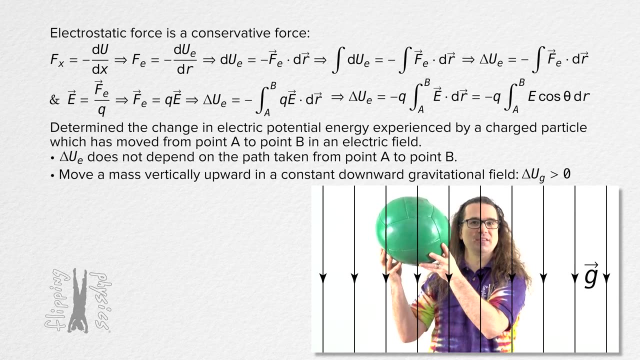 To make a comparison to gravitational potential energy. if we lift an object vertically upward in a constant downward gravitational field, it will experience a positive change in gravitational potential energy. In other words, I have increased the gravitational potential energy of this mass. Bo what happens if I let go of the mass? 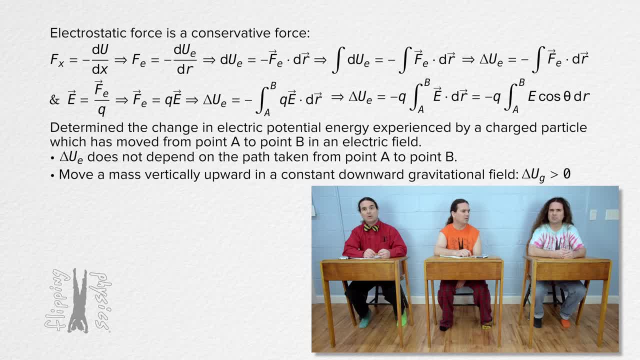 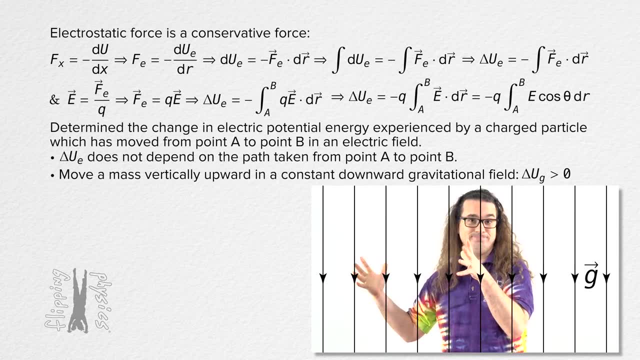 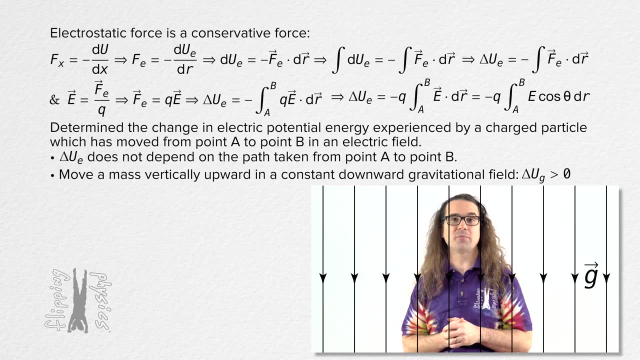 Uh, it goes downward, It accelerates downward, It accelerates in the direction of the gravitational field. Sure, Right, Conservation of energy says that gravitational potential energy of the mass will decrease and the kinetic energy of the mass will increase. And if we change the gravitational field to an electric field, 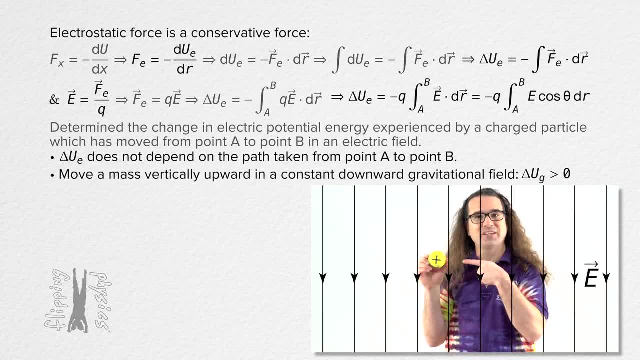 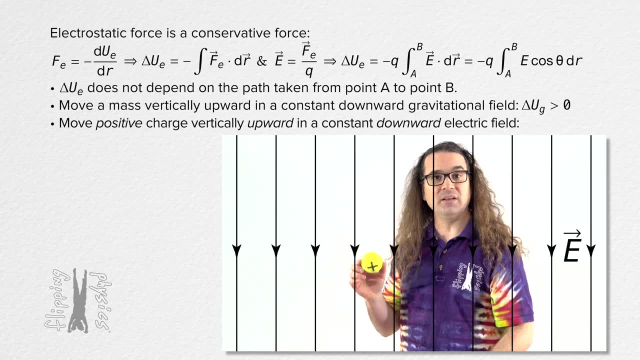 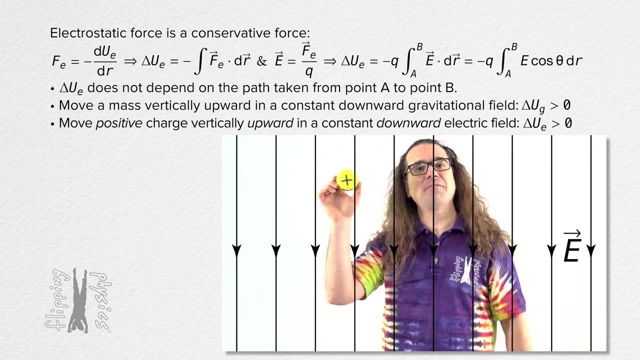 and use a positively charged object instead. notice that when we move the point A to point B- the positively charged object- opposite the direction of the electric field, it will gain electric potential energy, just like the mass did when I lifted it. And Bo what happens if I let go of the positive charge? 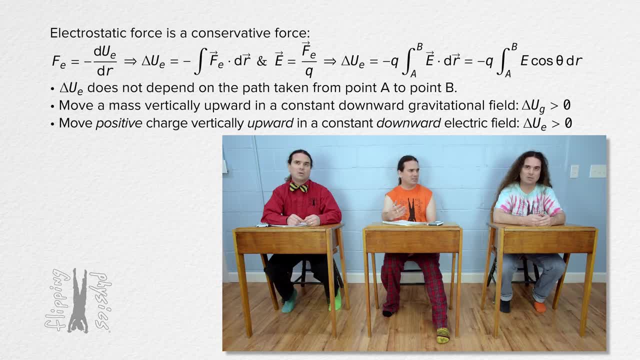 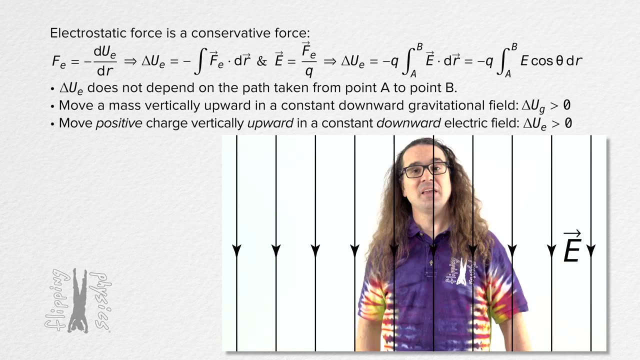 Uh, it goes downward, It accelerates downward. It accelerates in the direction of the electric field. Sure, As the electric potential energy of the positive charge decreases, it gains kinetic energy, Exactly Now, if I change the charge to a negative charge, 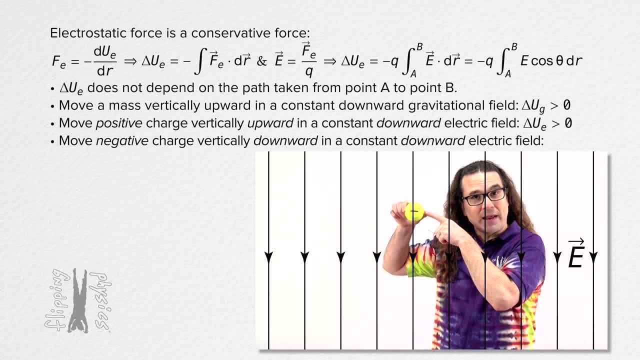 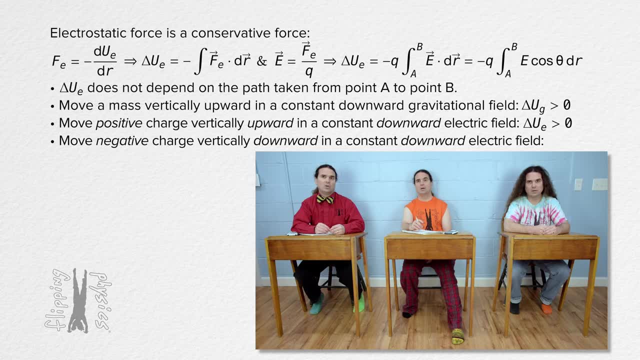 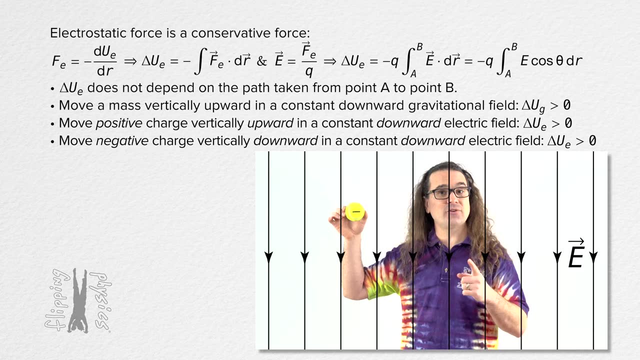 as I move the negative charge, this time in the direction of the electric field, Bo, what happens to the electric potential energy of the charge now? Uh well, it actually increases, right, Correct, Bo. If I move a negative charge in the direction of the electric field, it gains electric potential energy. 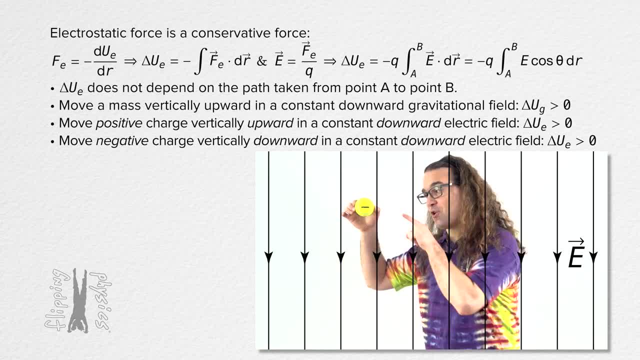 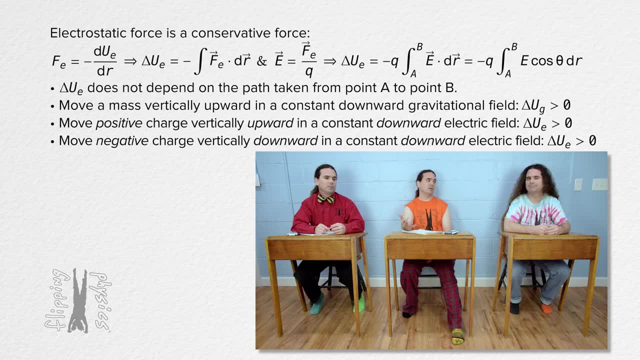 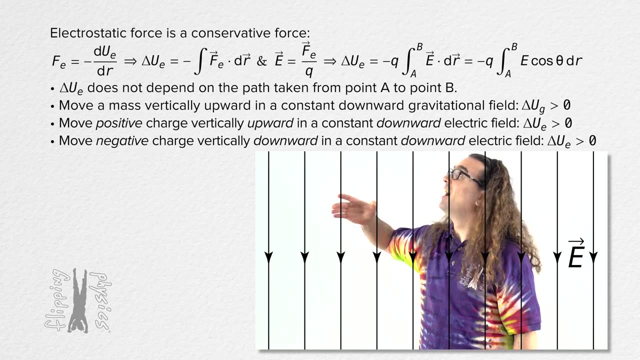 And class. what happens if I let go of the negative charge now? Uh, it goes upward, It accelerates upward, It accelerates opposite the direction of the electric field. Sure, Exactly Nice. I love this demo. Did you do that? 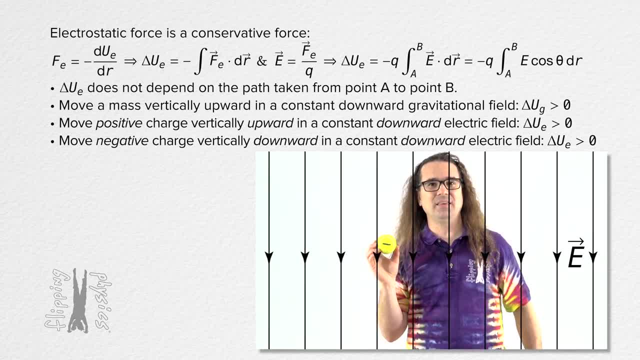 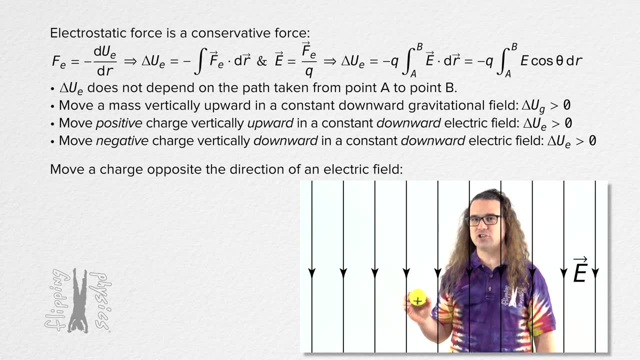 I do want to point out the negative and the dot product in the equation As I move the charge in a direction opposite the direction of the electric field. the direction of the displacement of the charge and the direction of the electric field are opposite to one another. Therefore the angle. 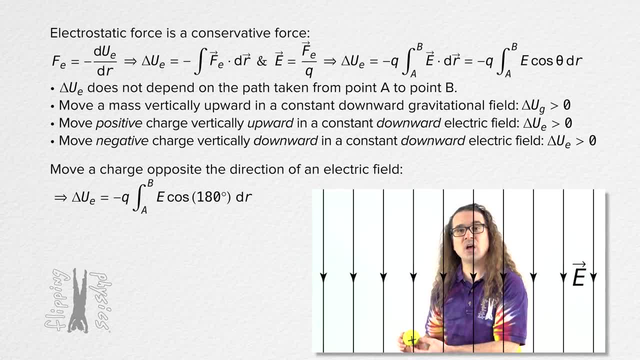 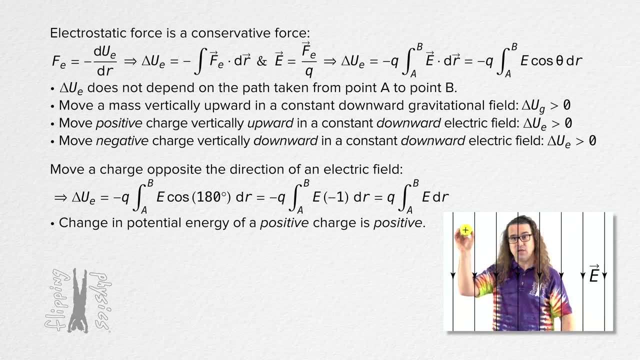 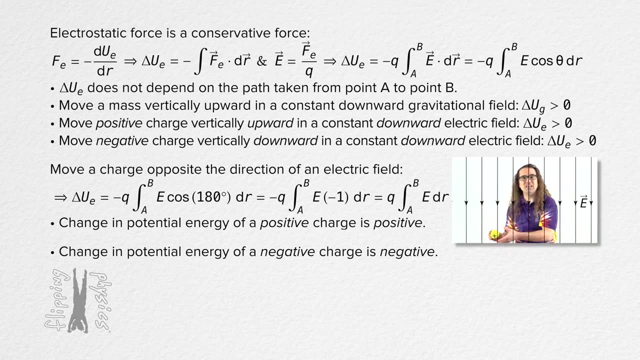 between those two directions is 180 degrees. The cosine of 180 degrees is negative one, which makes the change in potential energy of a positive charge positive and the change in potential energy of a negative charge negative. In other words, the electric potential energy of a positive charge increases as a. 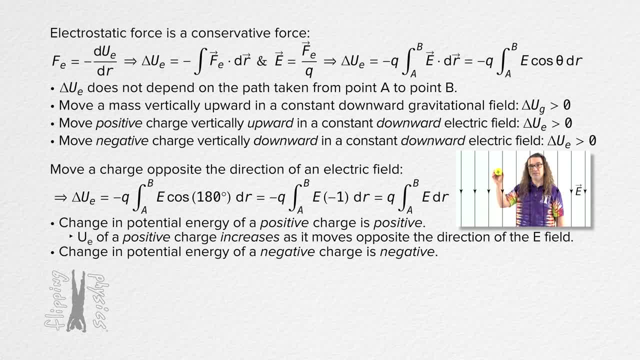 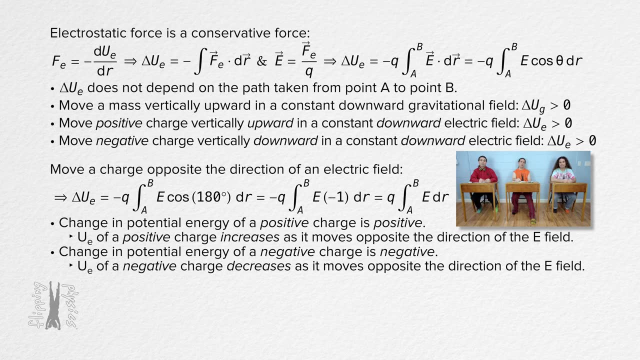 positive charge moves opposite the direction of the electric field and the electric potential energy of a negative charge decreases as it moves opposite the direction of the electric field. Realize there is no gravitational analogy to negative charge, There is no negative mass. So we are not used to this concept of the change in potential energy. 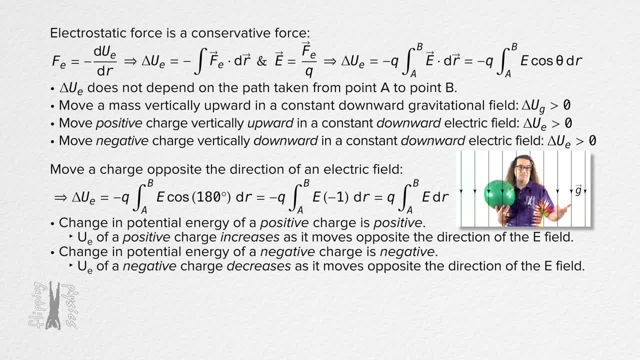 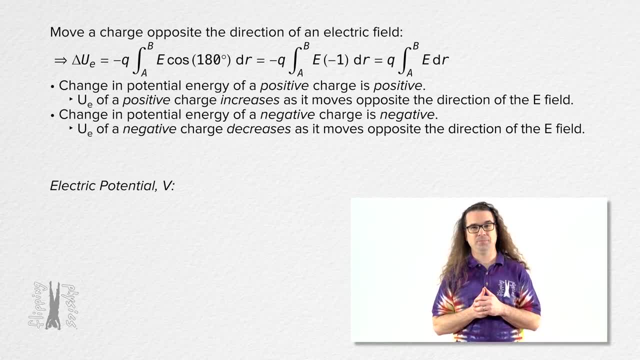 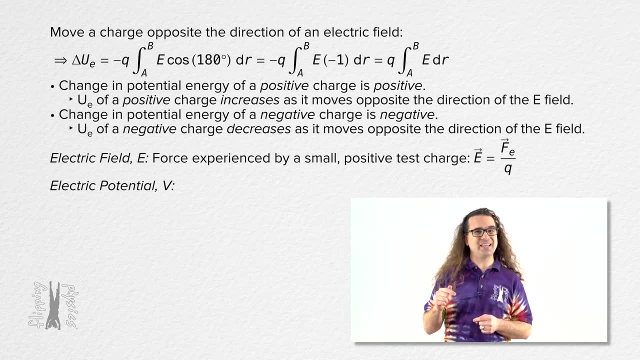 depending on whether the charge is positive or negative. Right, There is no such thing as negative mass. Next, we need to define electric potential. Just like we define electric field in terms of the force experienced by a small positive test charge, we define electric potential in. 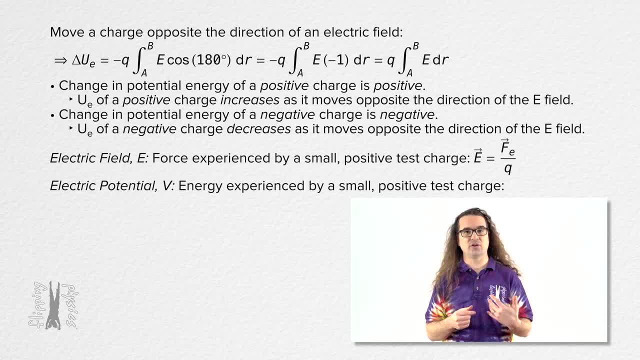 terms of the energy experienced by a small positive test charge. Electric potential equals electric potential energy divided by charge. The units for electric potential are joules per coulomb or volts. The symbol for volts is a capital V. I know the symbol for electric potential is a capital V. 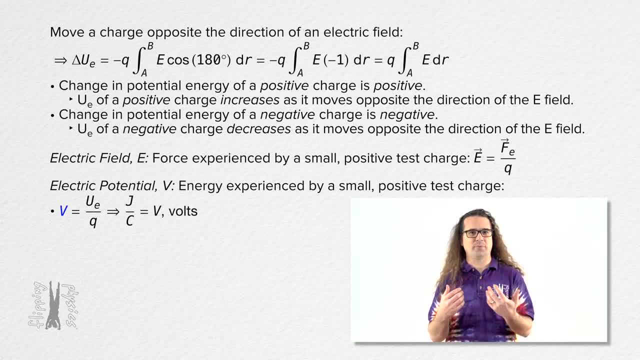 which is the same as the symbol for the units for an electric potential volts. This is not my fault and I don't know whom to blame. However, it is definitely not me. Grumble, Grumble, grumble, Grumble, grumble. 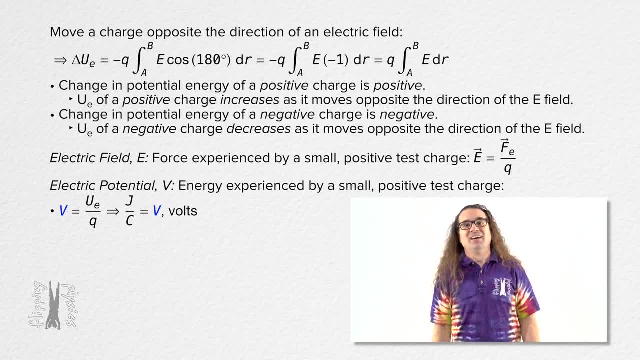 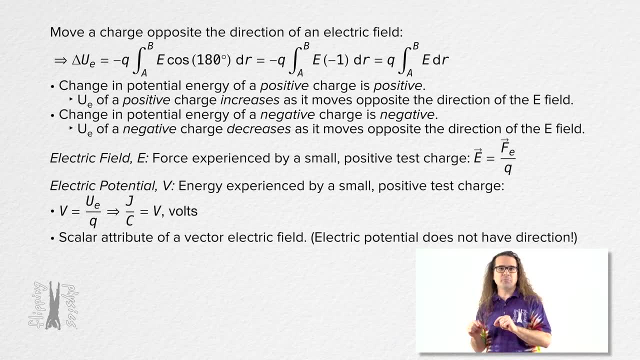 Aha. electrical Electric potential is a scalar attribute of a valvular electric field. In other words, the electric potential does not have direction. This fact that electric potential is a scalar can be very helpful in this class. I'll actually demonstrate that later in this lesson. 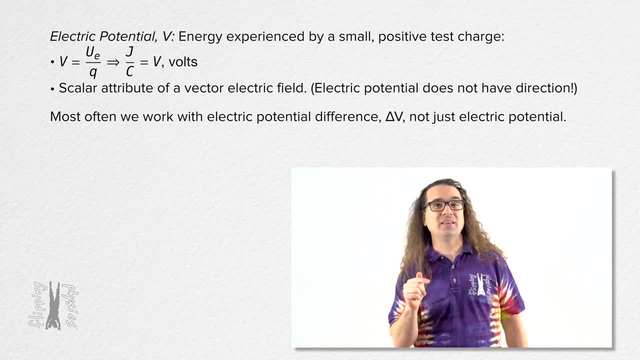 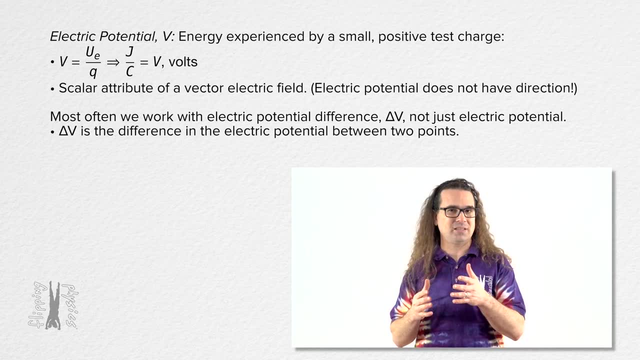 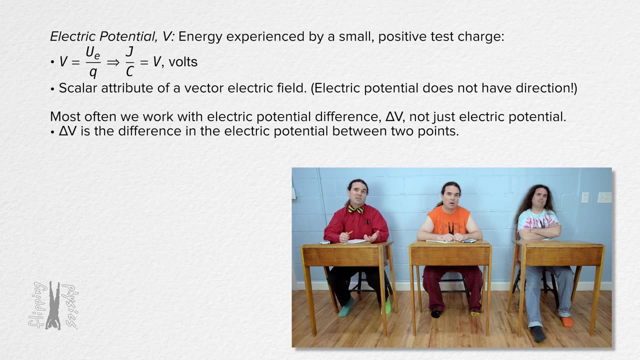 Now, most often we are interested in the electric potential difference, not just electric potential. Electric potential difference is the difference in the electric potential between two points. Uh yeah, It could be called change in electric potential, but we call it electric potential difference. 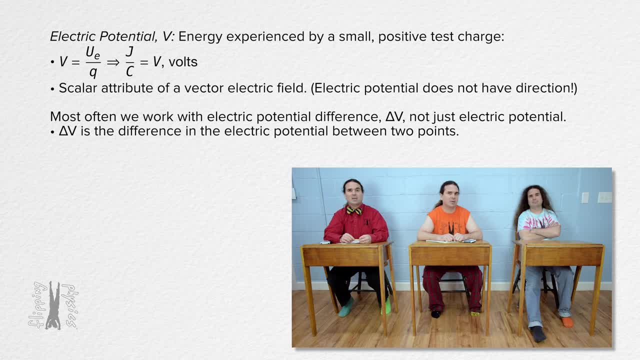 Actually, electric potential difference is better because it is a difference in the electric potential values at each location, regardless of whether a charge actually moves through that difference or not. So nothing has to go through a change in electric potential. The electric potential difference is just always there. That actually makes sense. Thanks. 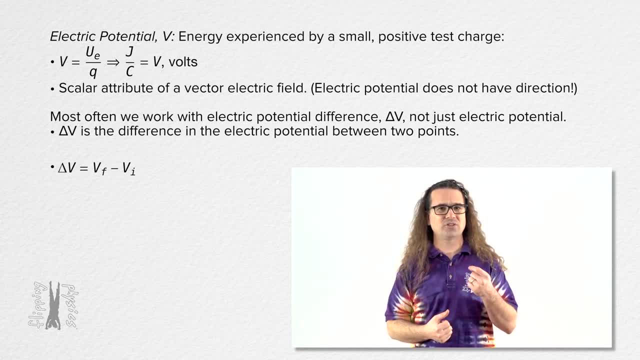 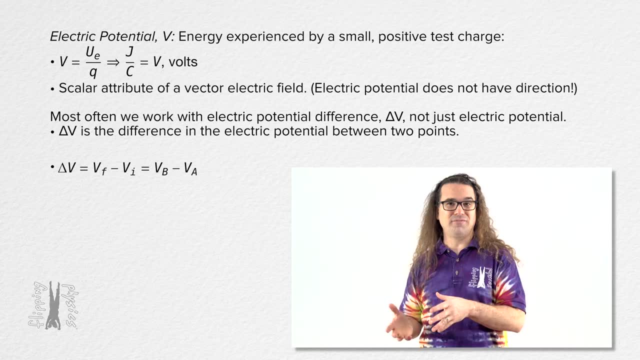 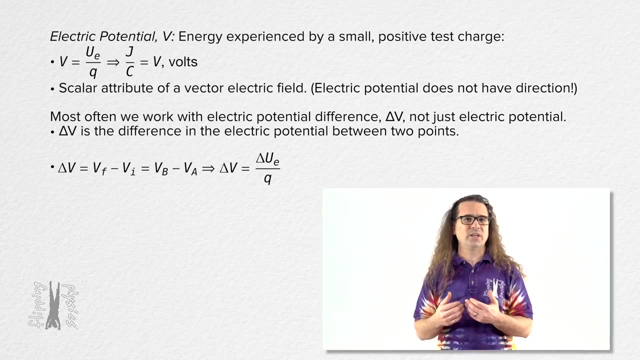 Right. Electric potential difference equals electric potential final minus electric potential initial. Often points A and B are used instead of initial and final. That means electric potential difference equals change in electric potential energy divided by charge. We can substitute the dot product integral equation in for change in electric potential energy and the charge cancels. 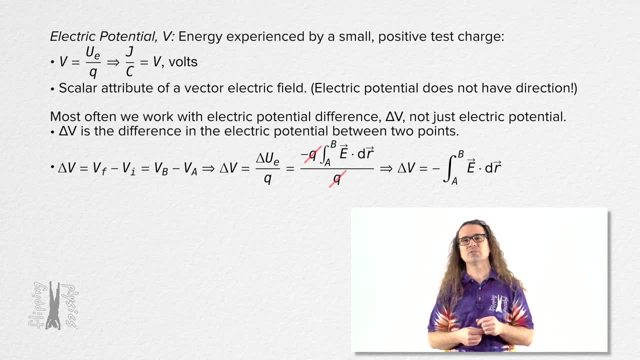 out And we are left with electric potential difference equals the negative of the integral from point A to point B of the dot product of the electric field and the infinitesimally small displacement dr. We will often set the initial electric potential or electric potential at point A equal to zero. 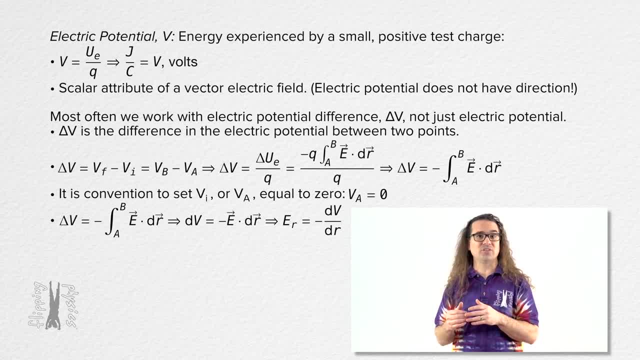 Notice, we can now essentially go in the opposite direction than we did at the very beginning of this lesson. We can go from the integral to the derivative And we get that the electric field in the direction of r equals the negative of the derivative of electric potential with respect to r. 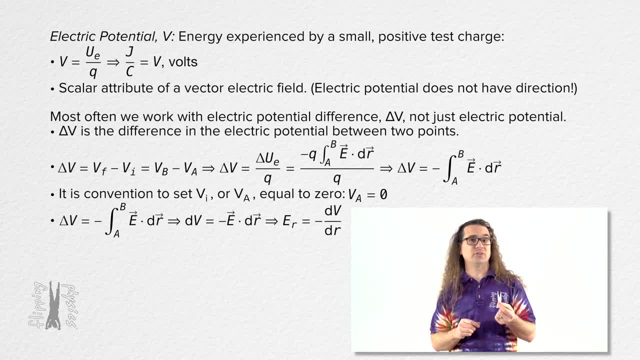 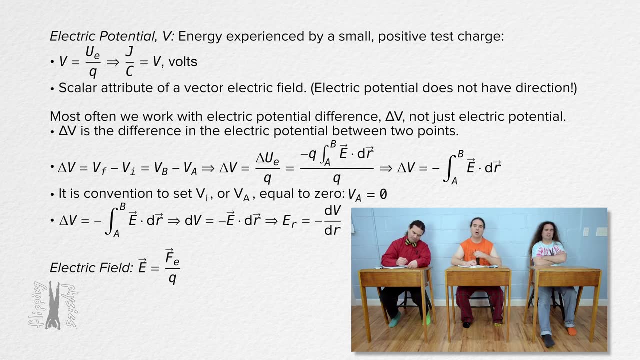 Okay, now that we have the electric potential units of volts, let's take another look at the units for the electric field, Bo. what are the units for the electric field? Well, electric field equals electrostatic force over charge, so the units are newtons.